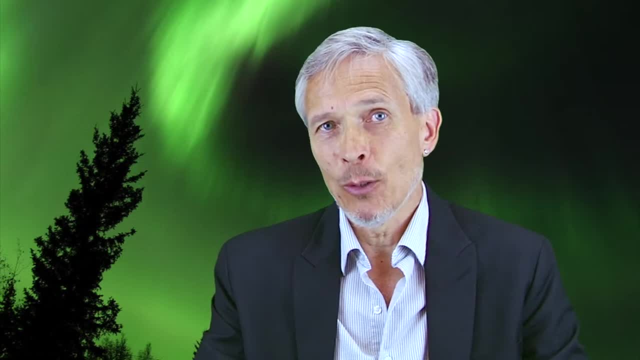 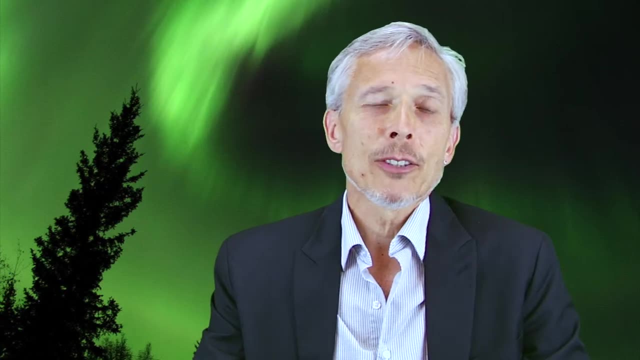 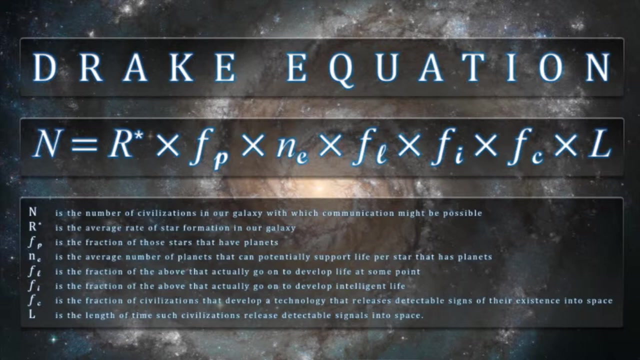 billion for the number of intelligent, communicable civilizations, But we assume that those are mostly at distances far too far to even imagine communication. What are the factors of the Drake equation? The first factor is the rate at which new stellar systems that could host planets are being formed in the Milky Way, the star formation. rate of sun-like stars. This number is a few- 3 to 5, and it's well determined by astrophysics. The next number is the fraction of those stars that have planets of any kind. Exoplanet searches are pinning this number down. 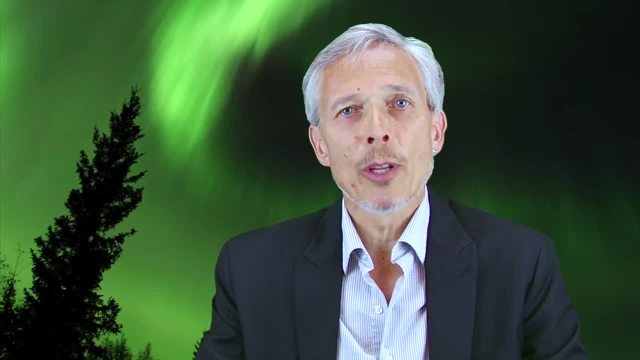 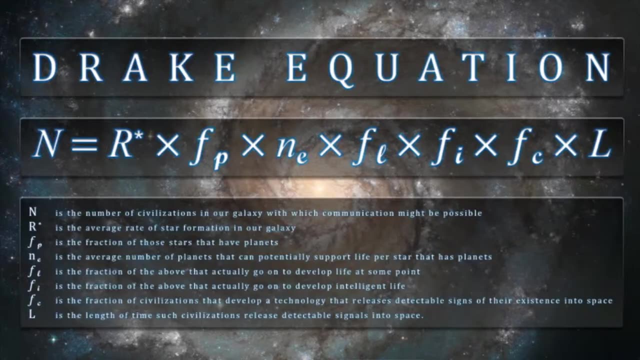 This fraction is going to be close to 1.. Already it's known to be more than about 20 or 30%. The third number is the number of Earth-like systems within each exoplanet system. This is the subject of intense investigation in astrobiology. We don't know the answer, but 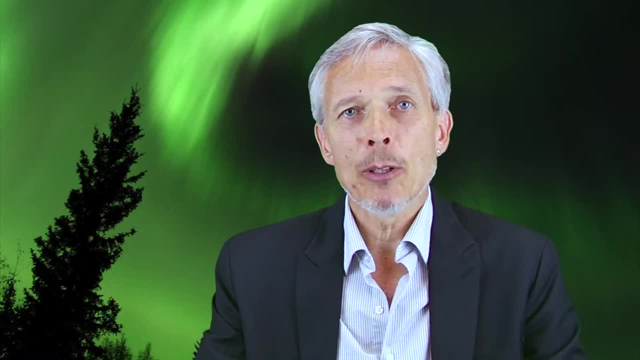 it's looking like N is 1 or 2.. There are typically a couple of Earth-like planets in each solar system out there. These numbers are all either determined or about to be determined by astronomical observation. The next factors will recognize as the number of planets that are being formed in the Milky. 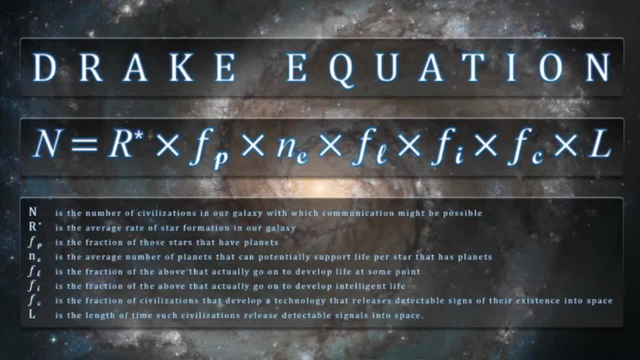 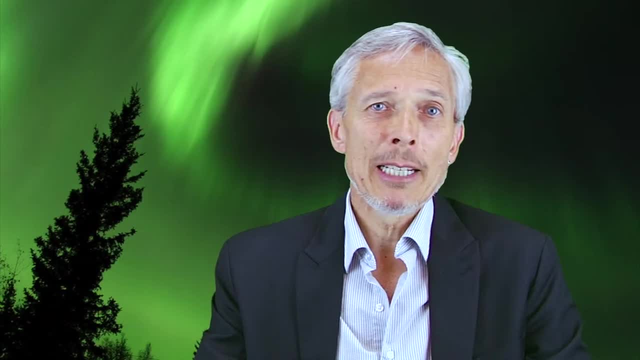 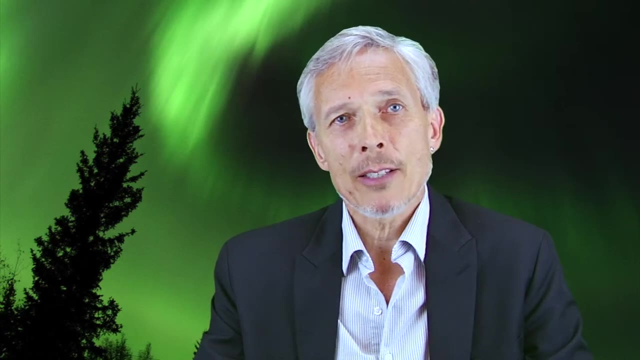 Way. The next one is the fraction of those Earth-like planets that have life. We don't know what that fraction is. We might imagine if a planet is habitable, it's almost inevitable that it has life, and so that fraction is close to 1. But some biologists argue that that's 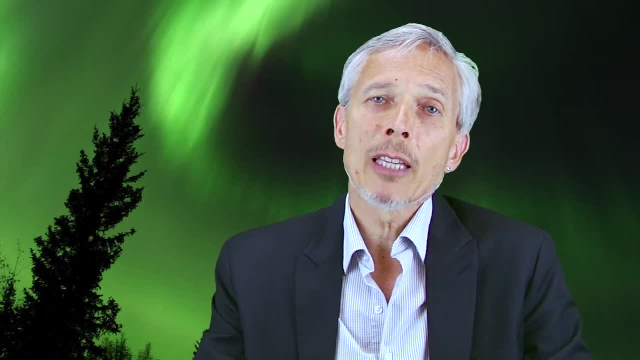 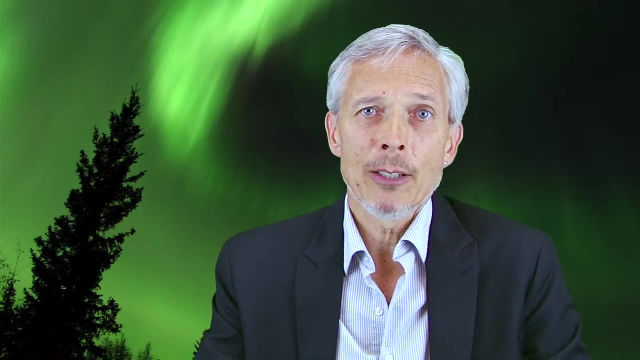 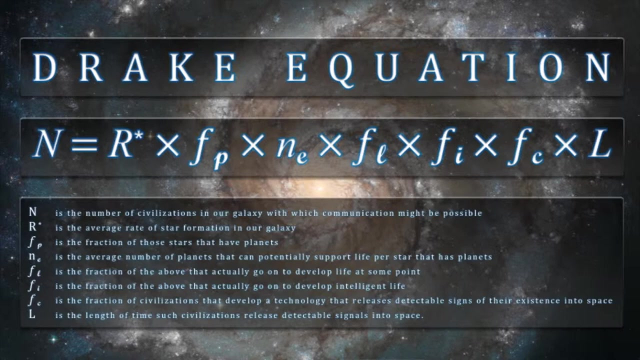 not the case that life's formation on the Earth involves some unlikely steps, and so that fraction is small, maybe only 1% or less. We don't have the data to decide until we find life elsewhere and get some statistical proof. The next fraction is the fraction of those planets where life forms, where an intelligent 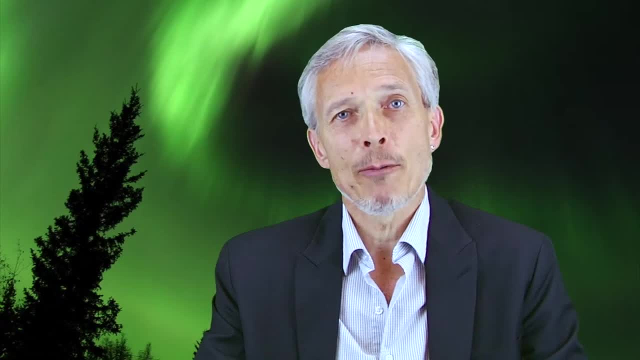 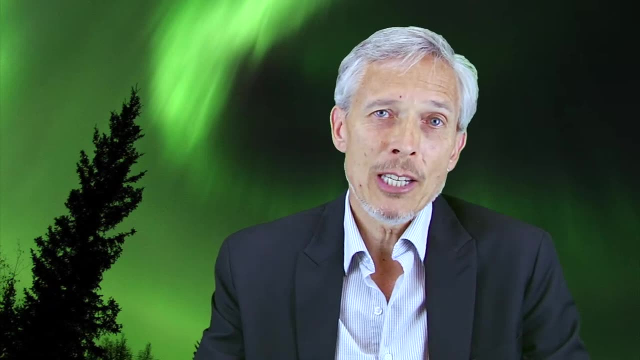 species eventually develops. Again, we have no idea of that fraction. Some argue that it's inevitable because it happened here. Others argue that it took a long time or it involves a lot of contingency and evolution and so it's a low number. There's no way. 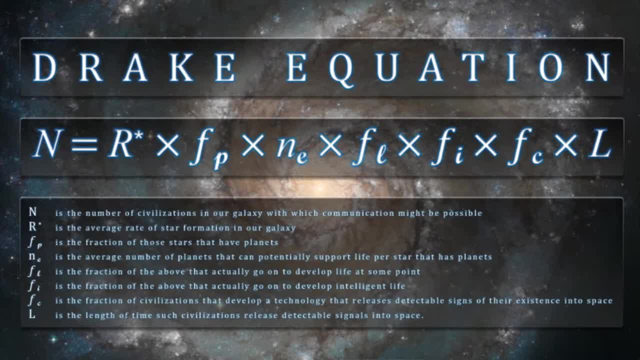 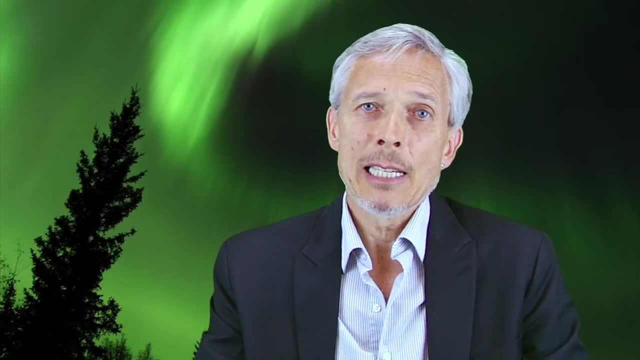 to decide. The next to last fraction is the fraction of those intelligent species that develop the ability to communicate or travel in space. On the Earth we have a handful, at least, of intelligent species that develop the ability to communicate or travel in space. On the Earth we have a handful at least of intelligent 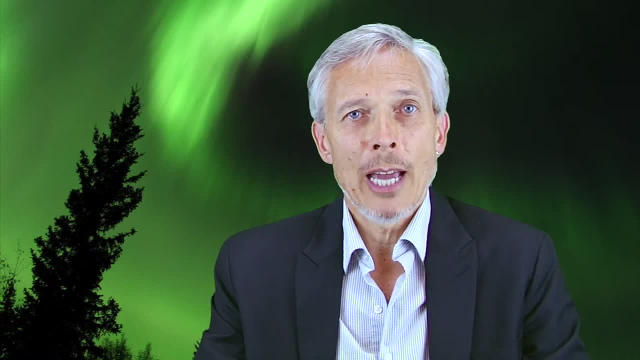 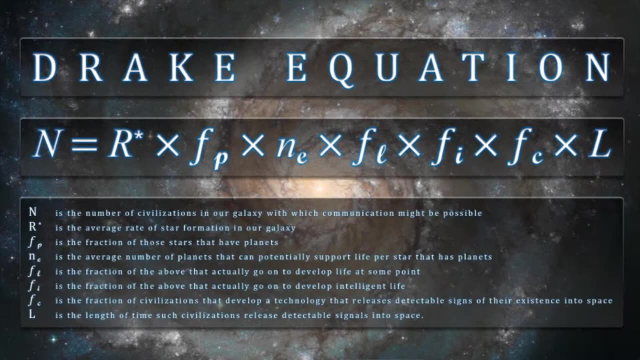 species that develop the ability to communicate or travel in space, Only one of which us has the ability to do that. But again, we have no idea what that fraction is. in the general case. The final number is critical because it involves time. It's the lifetime of that hypothetical 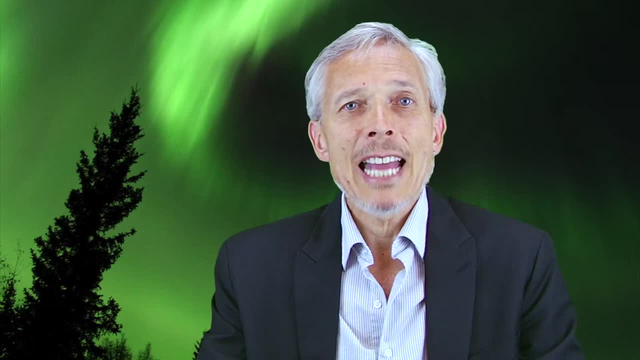 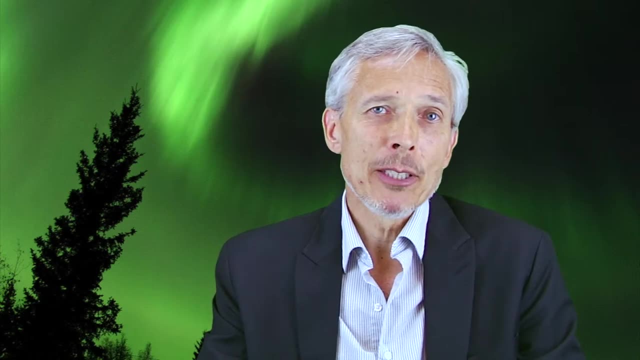 civilization in their communicative state. Since n is proportional to L, the entire product is driven by L. If L is a small number, then n may be a small number. If n is large, n may be large. What is L? 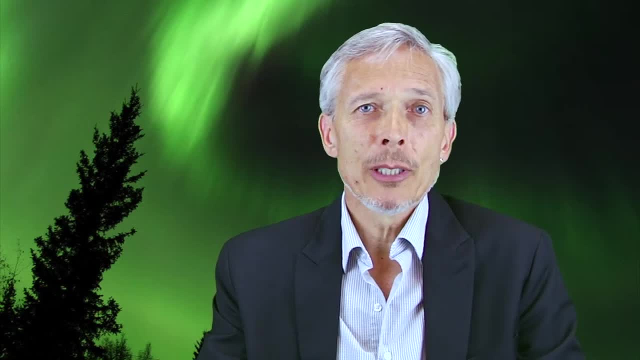 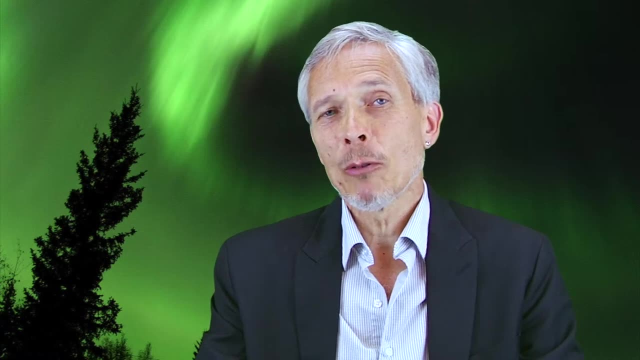 For us it's hard to tell We've only had the communication ability in space or to travel for 50 years, say 100 as a round number. but people looking at human history will realize we nearly extinguished ourselves in that time when there were 40,000 nuclear weapons in the world and the Cold 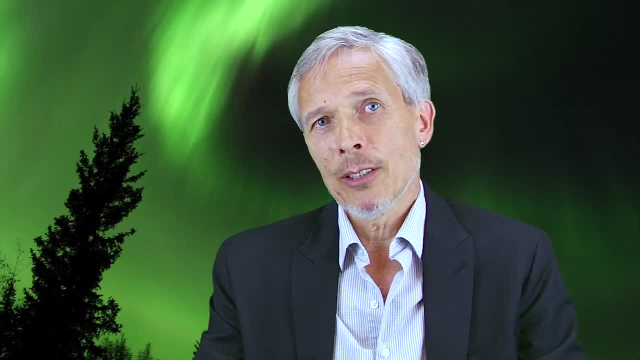 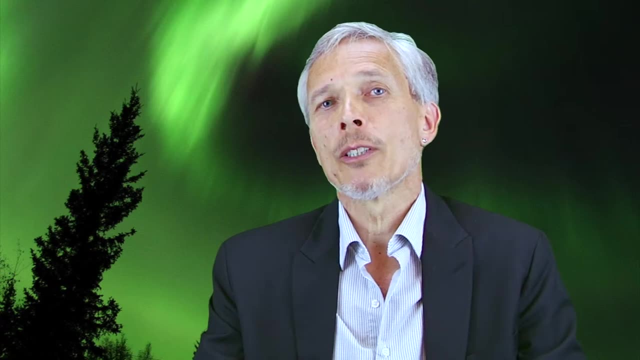 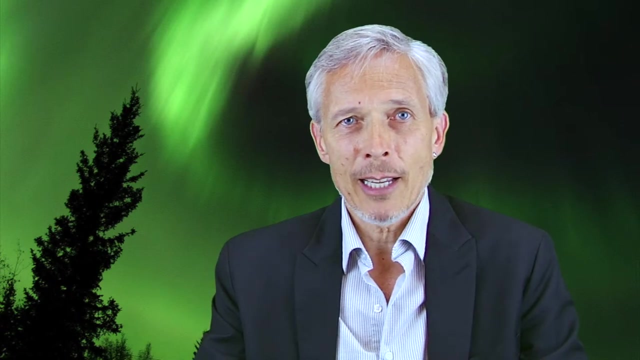 War was in its darkest days. So if human civilization, with intelligence and technology, is unstable, we don't know what the cosmic average of this number is. Perhaps civilizations always are unstable, or perhaps we're the exceptions, the immature ones who almost self-destructed. and when you get through your teething adolescence, 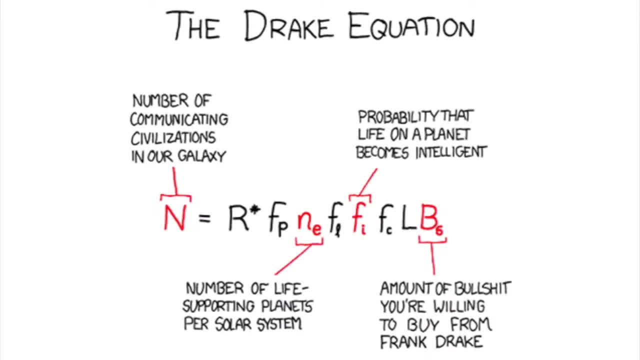 you live forever or for millions of years. You can see the huge uncertainty in the Drake equation and it's a simple trope of mathematics that the product of a series of numbers is as uncertain as the largest uncertainty. So the fact that we know the first three factors through astronomy increasingly well doesn't 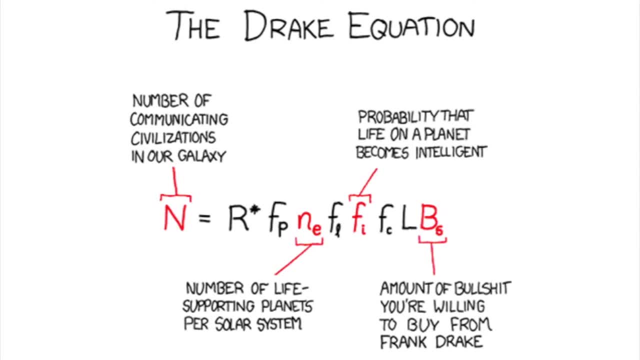 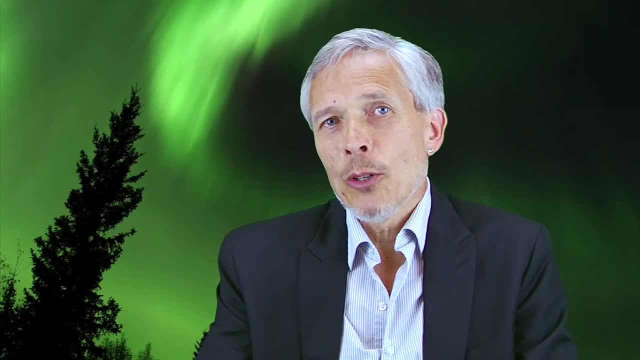 mean that the uncertainty goes away for the factors where we know nothing. Even Frank Drake recognized the limitations of his equation and he called it a container for ignorance. It is also worth pointing out, logically, that it's the number of intelligent communicable civilizations in the Milky Way. If some civilizations live a very long time, they could have the possibility to travel between galaxies At one-tenth light speed. the trip to Andromeda is perhaps 20 million years. For a nearly eternal civilization, this is not a long time and it's a small fraction. of the age of any galaxy. We're heading into extremes of speculation here, talking about the longevity of civilizations, But it's also important to point out that the Drake equation involves an average and that the possibilities of intergalactic civilization and communication may depend on the longest. 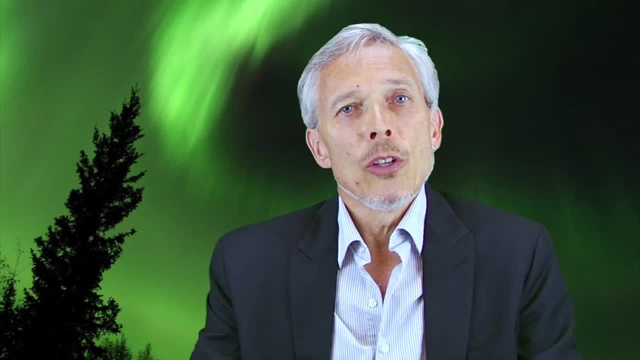 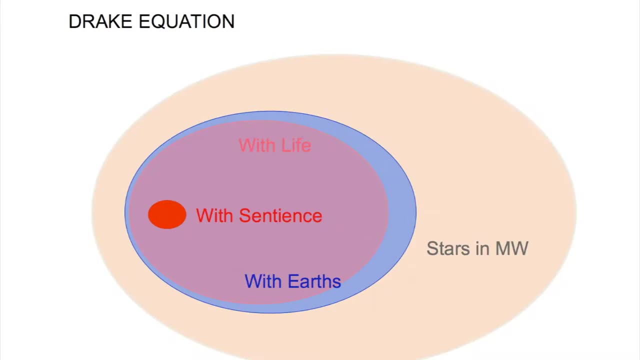 lived members of that club rather than the short-lived members. You can see that the Drake equation, conceptually, is a series of subsets. There's the subset of all the stars that have Earth-like planets, the subset of those that host life as opposed to the ones that are sterile or stillborn, and then the subset 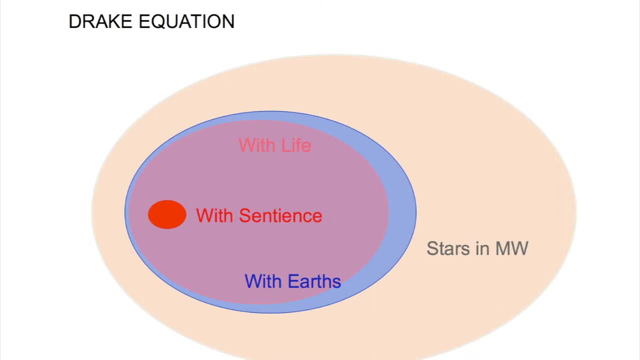 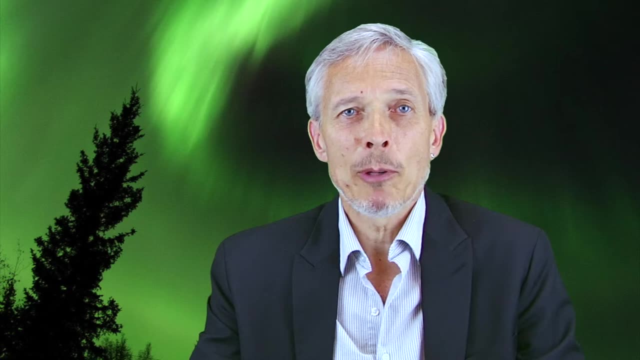 of those where life develops: sentience, And then intelligence and eventually technology. As we winnow down the very large number of sites for life, the initial real estate from the habitable planet searches, we could end up with a very small number. 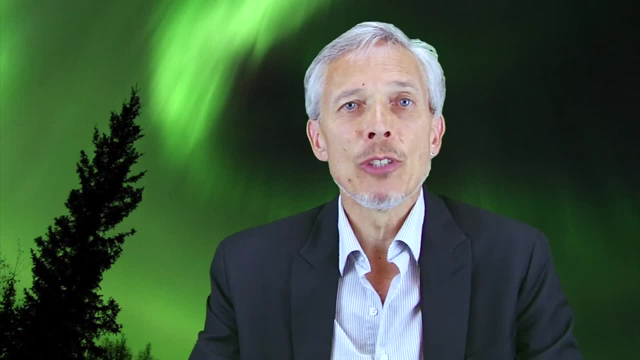 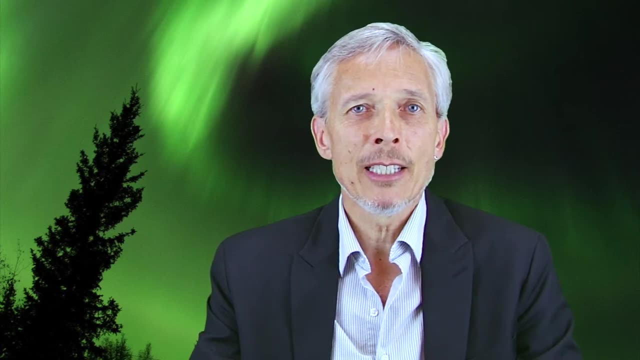 Logically, it's possible that N is one We're it. We're unique in the galaxy as an intelligent technological civilization. Also logically, and some have argued, like Carl Sagan, that N is more likely to be 100,000. 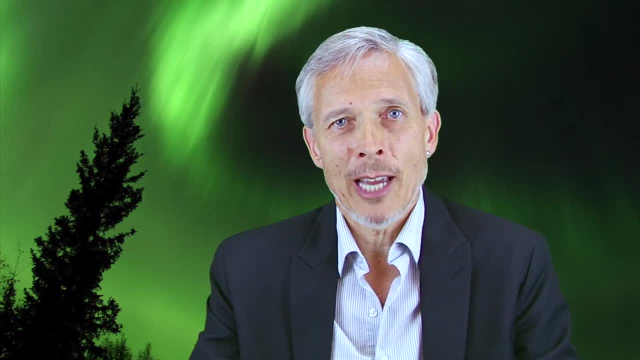 or a million, in which case there's a large set of potential pen pals out there: Sociologists, scientists, scientists, scientists, scientists, scientists, scientists, scientists, psychologists and evolutionary biologists have also weighed in on this subject. even 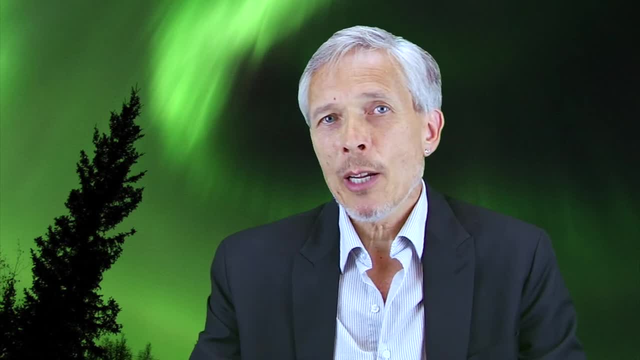 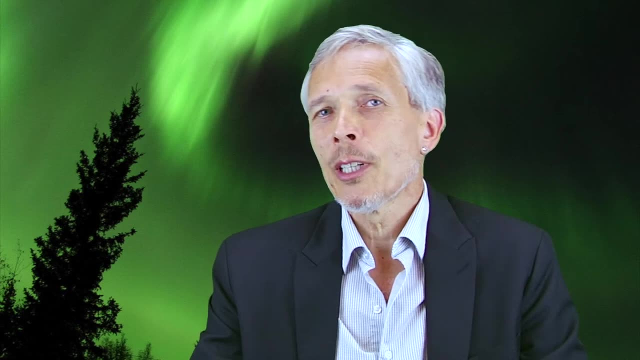 though it's mostly governed by astronomy arguments, Because when we're talking about the biological and cultural aspects of the equation, we have to do that kind of analysis of our situation. But the uncertainty of the Drake equation doesn't go away. In the end, we simply have to do the experiment and look. 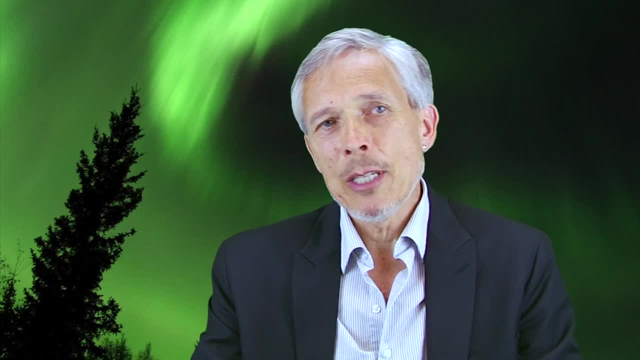 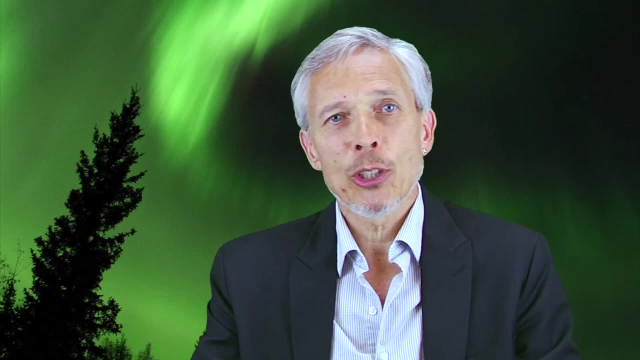 It's striking, and probably a coincidence, that Thomas Wright, a physicist living in England in the middle of the 18th century, speculated about the size of the moon. He speculated about the size of the Milky Way galaxy during a time when Herschel was. 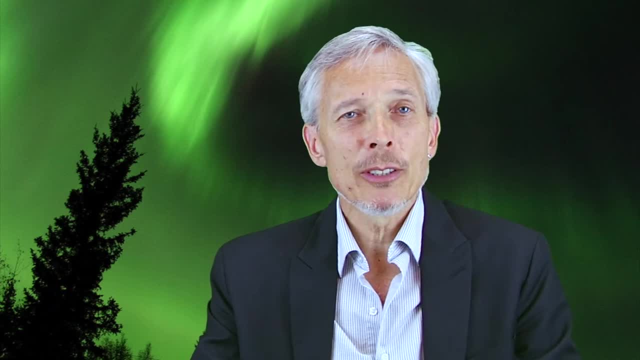 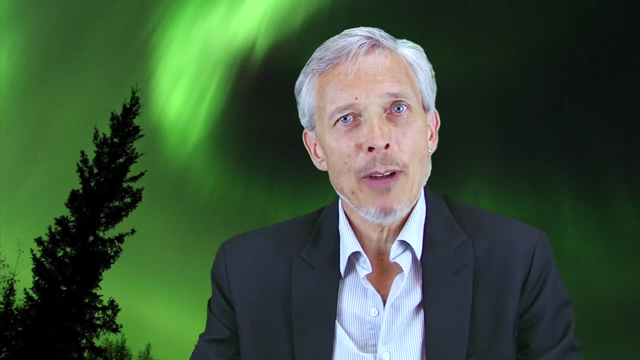 mapping it out with his telescopes and he came up with an estimate of 170 million habitable worlds in the universe, which at that time was the galaxy. This is actually close within a factor of two and certainly an order of magnitude. 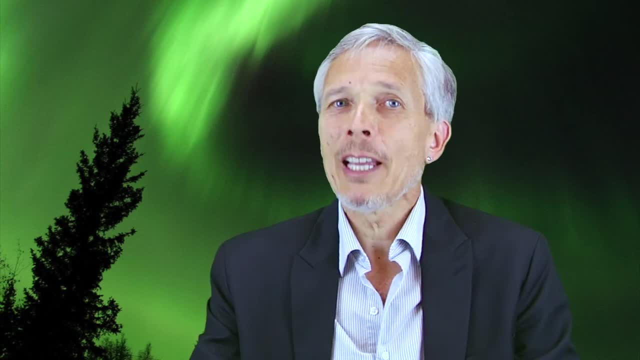 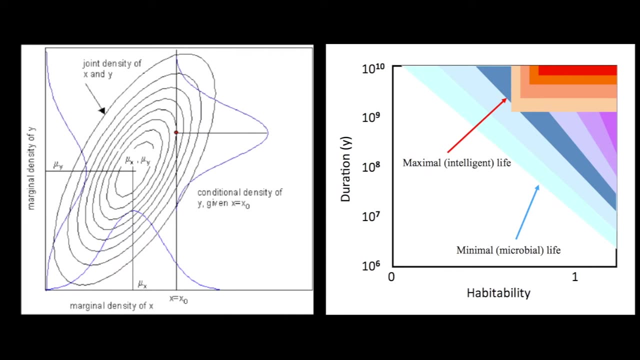 of the true modern astronomical estimate. So people have been thinking in these terms for centuries. There are more sophisticated ways of thinking about the Drake equation and there's a theoretical construct which stops using the binary On off. life exists or it doesn't. it's intelligent or it's not, and takes into account. 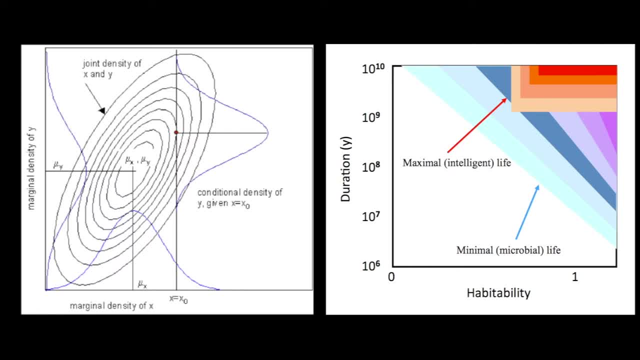 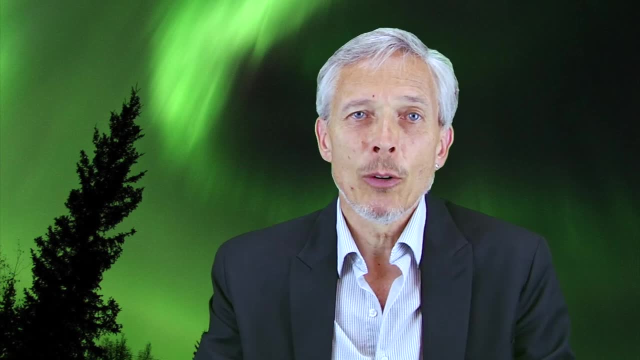 the contingencies of evolution and the fact that all of these attributes will exist on a spectrum and that some of the relationships between the factors are not independent. they're coupled. This is called a Bayesian framework for estimation. It's important that we use as few prior assumptions as possible in studying the Drake equation. 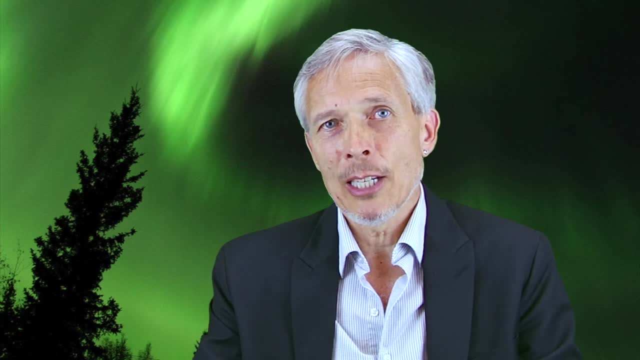 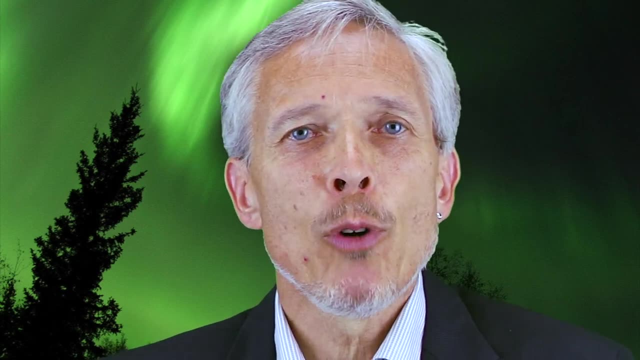 Either way, there's an enormous possibility for intelligent civilizations in the universe. The Drake equation seeks to organize the universe. The Drake equation seeks to organize the universe. The Drake equation seeks to organize our knowledge and our ignorance of astrobiology in one formalism. 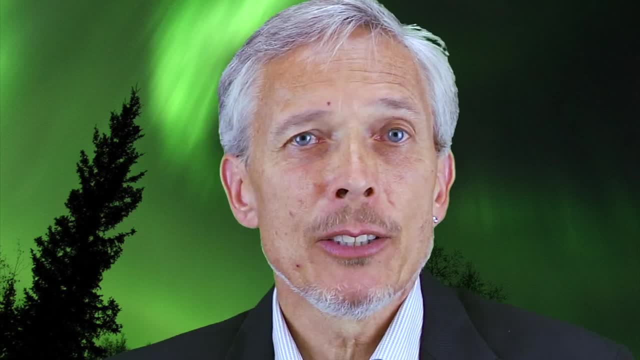 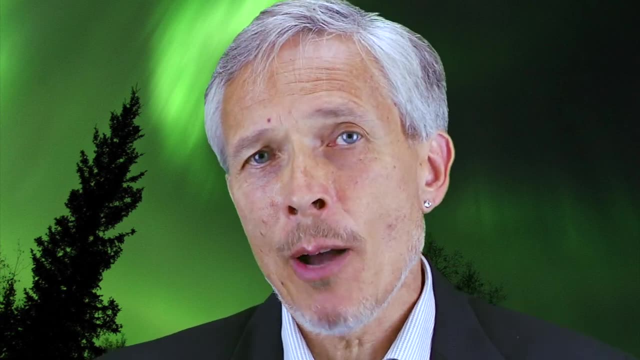 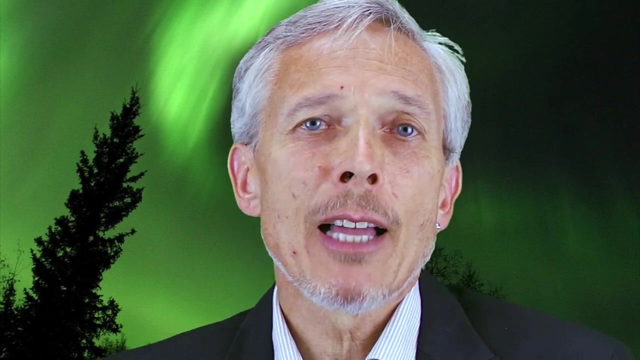 a simple equation to calculate n the number of intelligent communicable civilizations at any time in one galaxy hours. The first few factors of the equation are astronomical and they are being determined by current and future observations. The latter factors are completely uncertain because until we find life elsewhere, we won't.